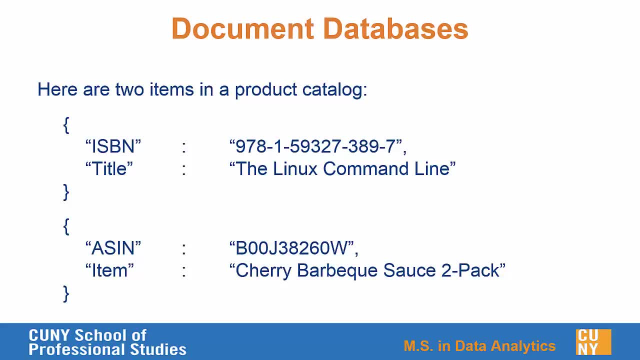 of documents that might be in a product catalog database. Notice here, though, while it's still very simple, it's got an identification number and it's got a title for the item. The rows don't have the same data structures. In the first case, we have an ISBN. in the 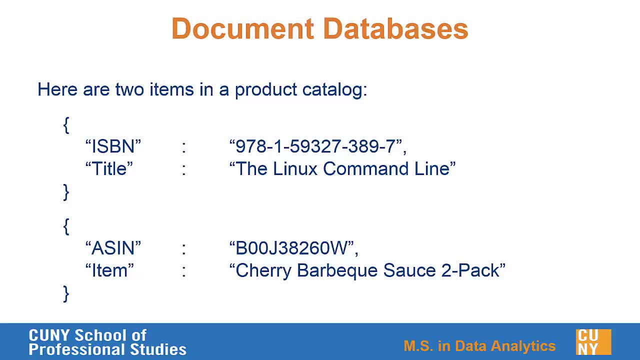 second case we have ASIN instead, So we're not required to have the same schema for each document. In the first case we have title, in the second case we have item. We can also store more complicated documents. So here's an example of a book with two authors. So 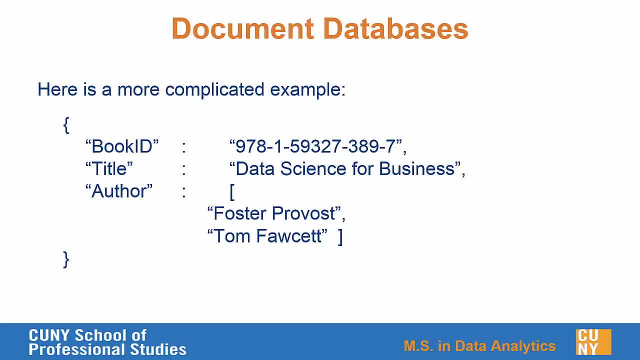 we have a book ID, we have the title and then in the key value pair for the author we have a more complicated object. We have a nested object. here We have two different authors, So document databases allow for more complex structure than just a simple row. 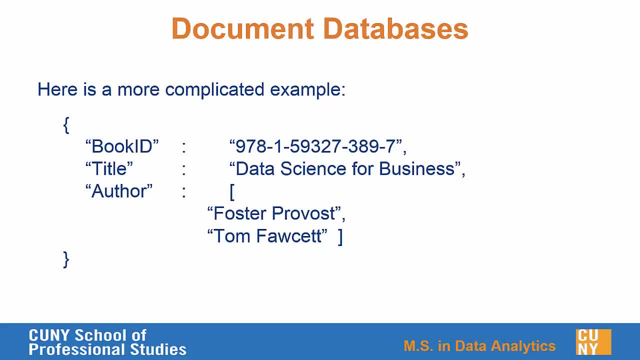 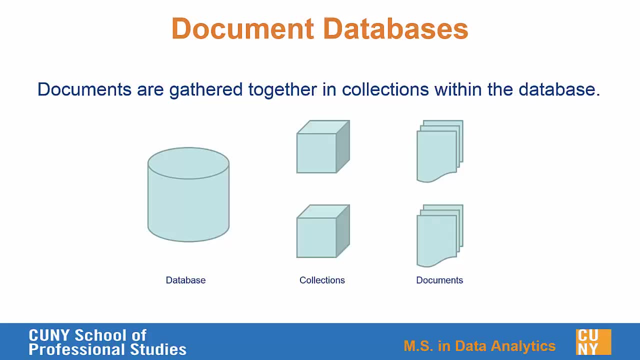 And we'll see examples of that throughout the various tasks that we give you for the course. So document databases are structured a little bit differently from SQL databases. In SQL you've got your database and then you've got your tables within the database. 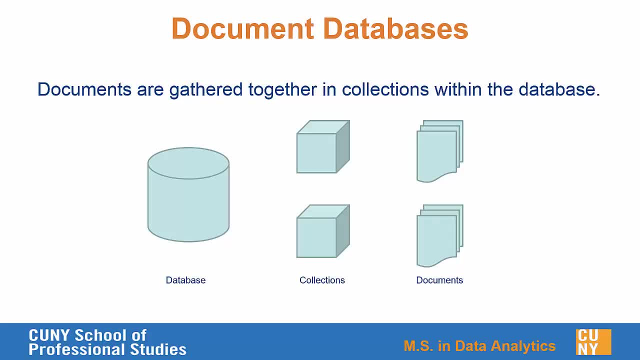 and then you've got rows within each table. So, similarly, in document databases, you have your database and then you have what we call collections, which are just groupings of documents, And then you've got within each collection. you can have any number of documents stored. 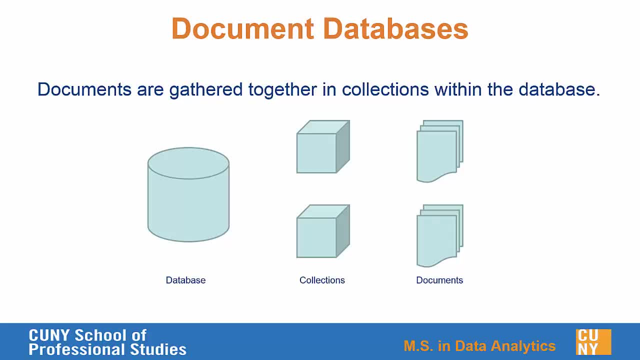 within that collection. Obviously, we like to choose collections that make sense. So one way to do things would be to have a books collections, have a videos collections, have a food products collection and to organize things in that manner. But you don't have. 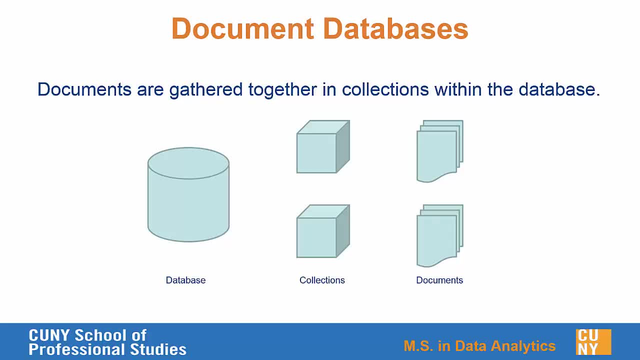 to do it that way. You could have a web store collection that has all of those different types of items in it, and then you could have a retail store collection, for instance, if you have different items available in stores and online. So there are a lot of different. 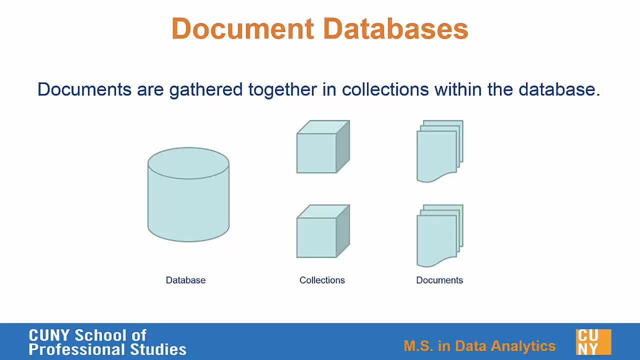 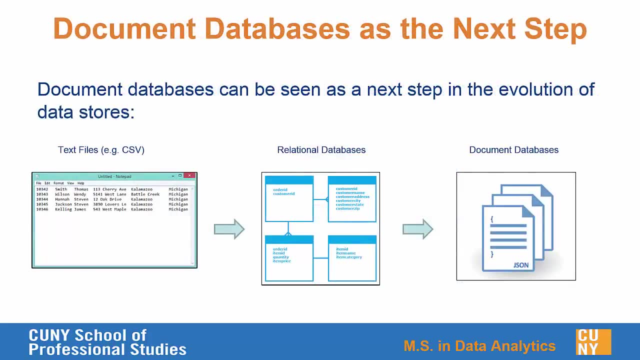 ways to structure your document database, And that's why we say document databases are fairly unstructured and schemaless. Document databases can be seen as the next step beyond relational databases. in a sense, You can see where the evolution goes from originally storing information in flat files.